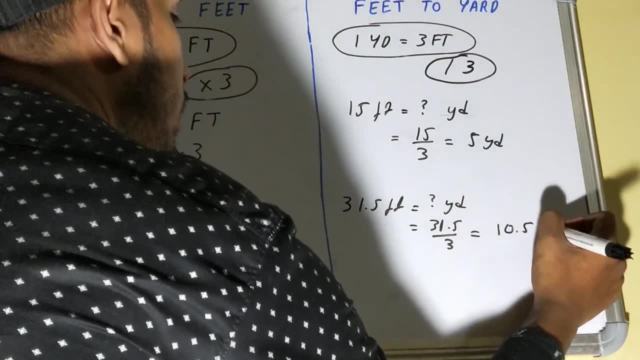 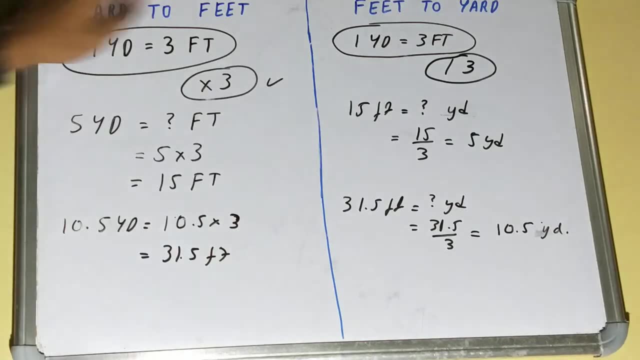 ten point five yards, so this is all you'll be finding. so this is very easy. for yard to feet, just multiply by three. for feet to yard divided by three. okay, so this was also. if you found the video helpful, please do hit the like button. do not forget to subscribe and thanks for watching. 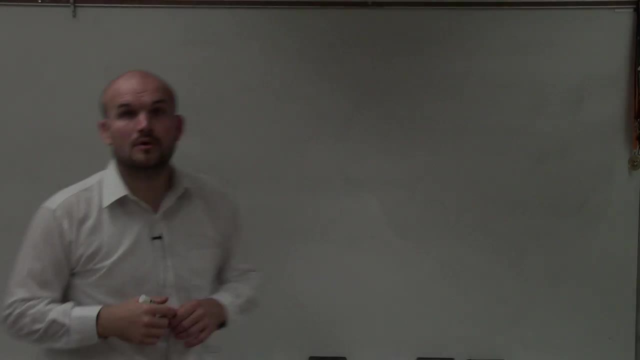 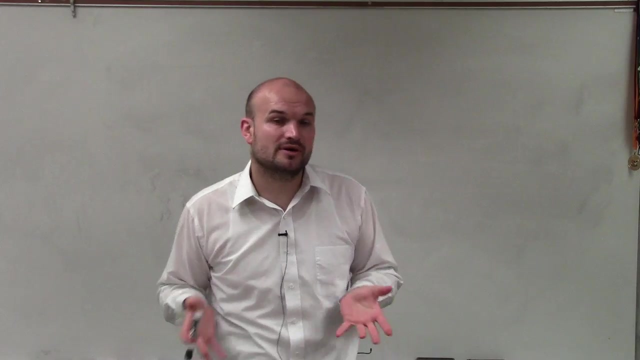 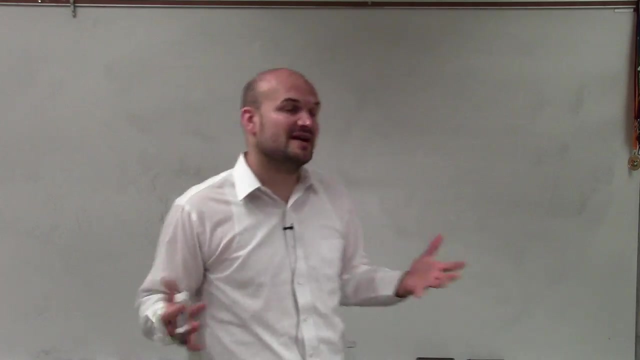 Welcome. So what I'd like to do is be able to explain to you what is the difference between a concave and a convex polygon, And this becomes very important as we start solving problems involving polygons that a lot of times we're going to need to have only convex polygons. 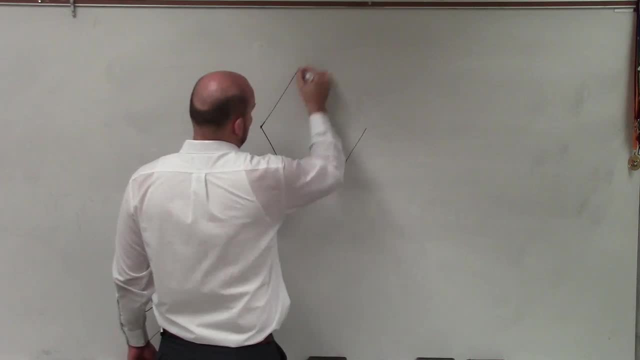 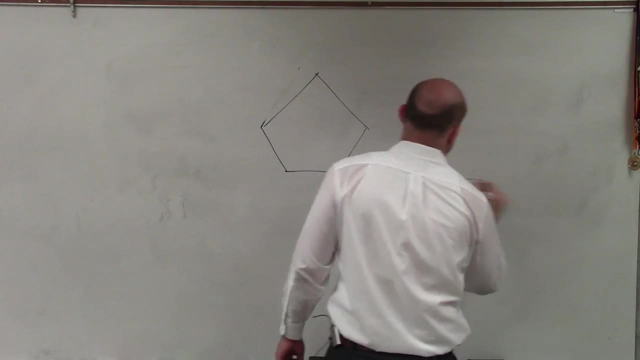 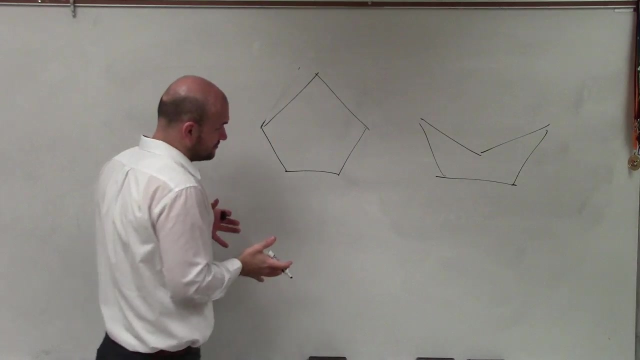 So what exactly is the difference? Well, let me kind of draw two polygons here. That's not the way I wanted to do it, OK, So you got one that looks like this, And then you have one that looks like this. So you can see, and they should have connected, right. 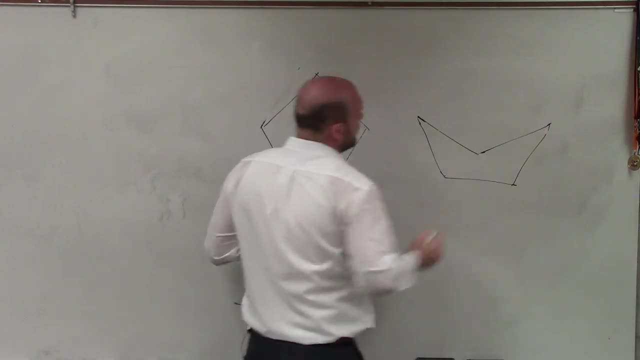 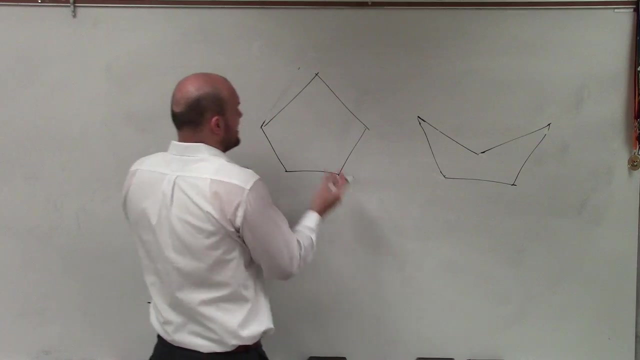 And they connect at their vertices. OK, So one thing, we there's a way that we can determine if it's convex or concave. But one thing you can kind of notice about these is all these vertices are kind of all out where on this one you 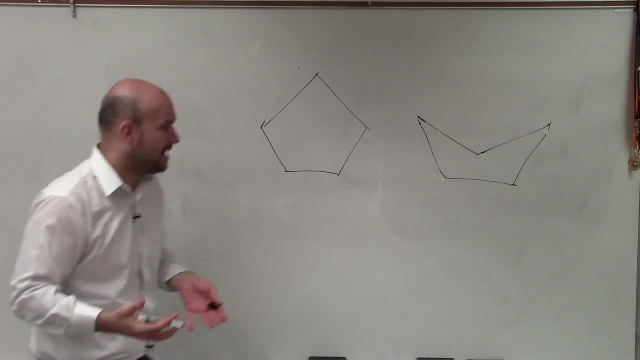 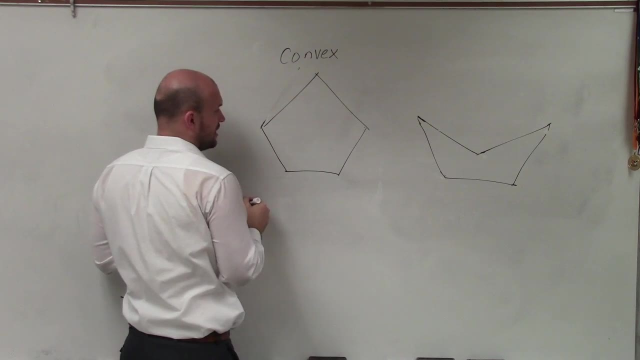 can see this vertices is kind of like pointed back in the polygon, And that's exactly pretty much the definition that we looked to When we have a convex. all right, the way that we can determine a convex is simply just extending all of the sides of a convex polygon And 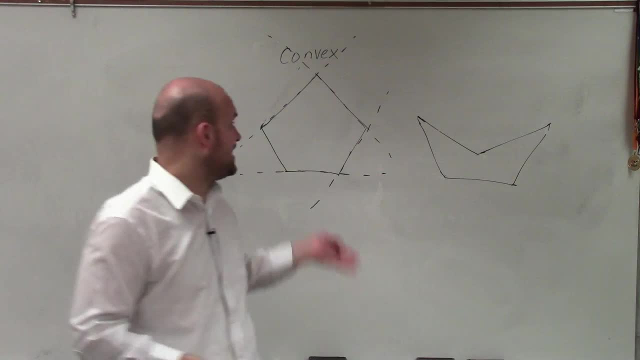 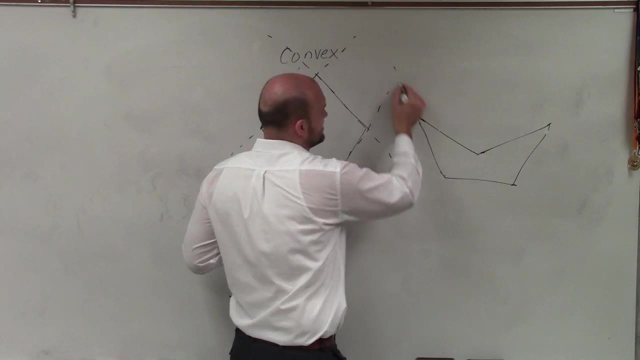 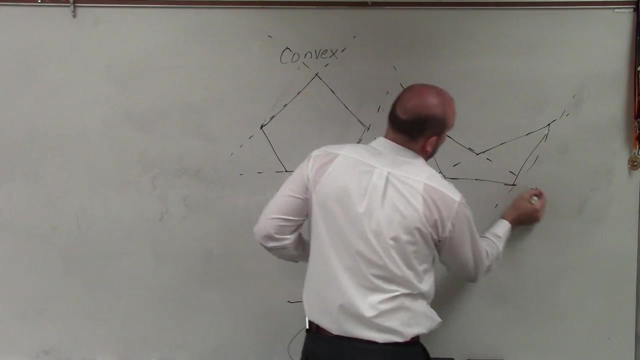 when I extend all of the sides of the convex polygon, you see that none of the sides intersect in the interior of our polygon. Therefore it's convex. However, when I do this with this concave polygon, what we notice is now the sides intersect when I extend them inside. 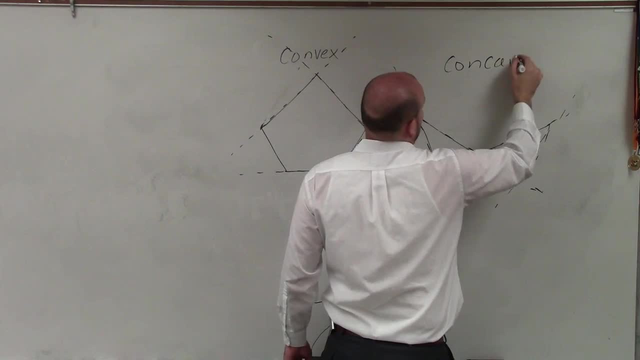 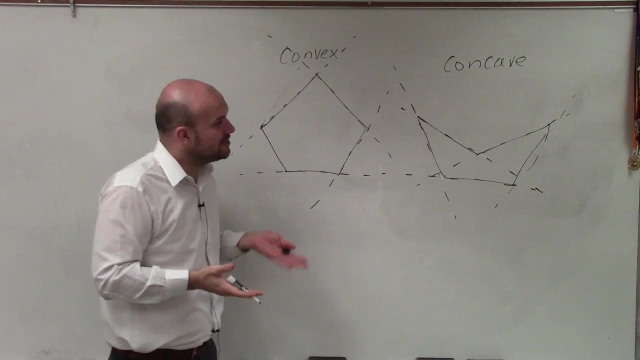 of the polygon. So this is what we call concave, And that's basically the understanding you can see. You know, think about it as a cave. You're kind of caving in to the polygon And that's going to be your basic way to be able to determine which one is which. And then 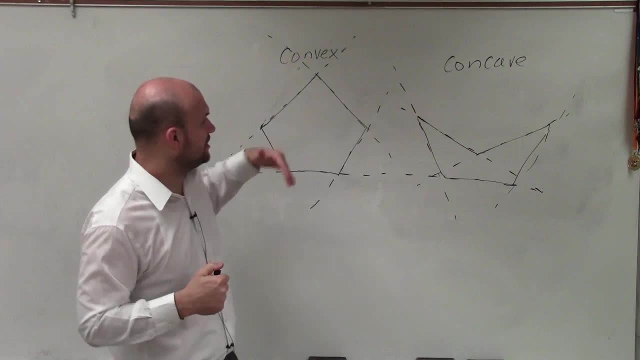 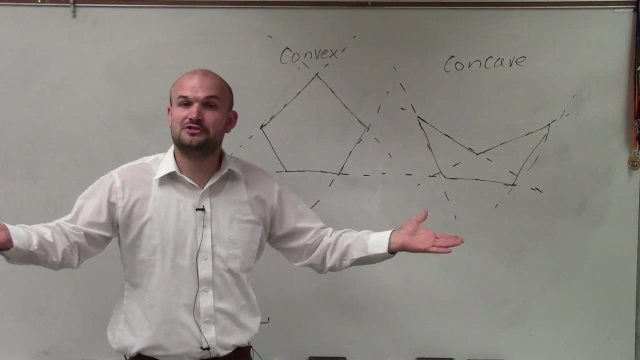 we'll get into further in the course of example of. you know how to determine between one or the other, As well as you know how we can use each one to be able to solve problems. So there you go, ladies and gentlemen. That is your basic difference between concave and convex.